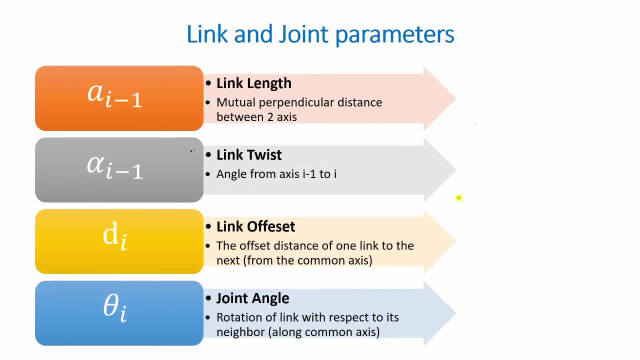 which make up our DH tables. Now these can be understood by considering two arbitrary joints. So let's just imagine a joint here, a revolute joint, connected through some sort of link to another revolute joint over here. Now each of these joints would have their 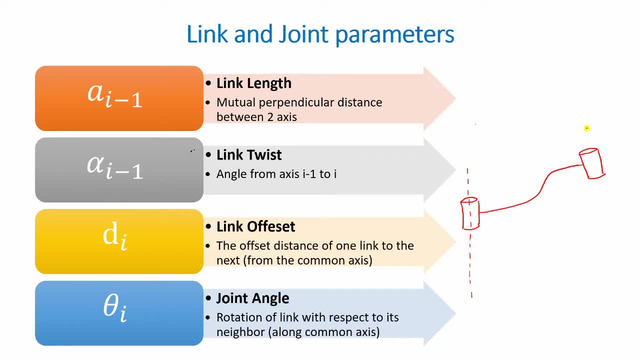 joint axes. right, so the first value is our ai minus 1, which is the link length. for this it would be the length of the common perpendicular between both these two axes. so that would be your ai minus 1. your second parameter would be the link twist. so if you assume this joint to be our ith joint, 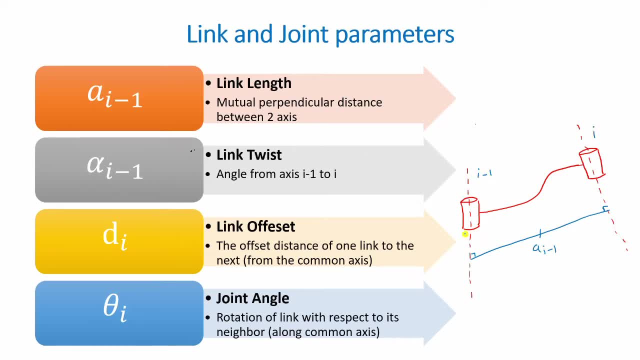 this would be our I minus 1, so this axis can be redrawn over here or something like that, and this angle would be our link twist alpha I minus 1. the third value is the link offset, which is the offset distance between the link and the common axis, so sort of something like this: and T to I. 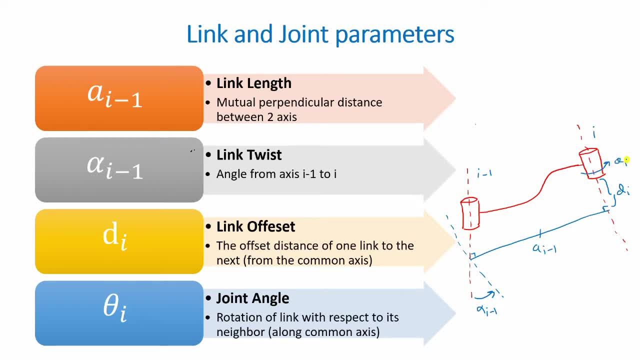 would be the rotation of the joint. so typically, di values will only exist for prismatic joints because they move linearly up or down, left or right, while T to I values will usually exist only for revolute joints as they revolve around a particular axis, which means revolute joints should have a 0 di, while prismatic values should. 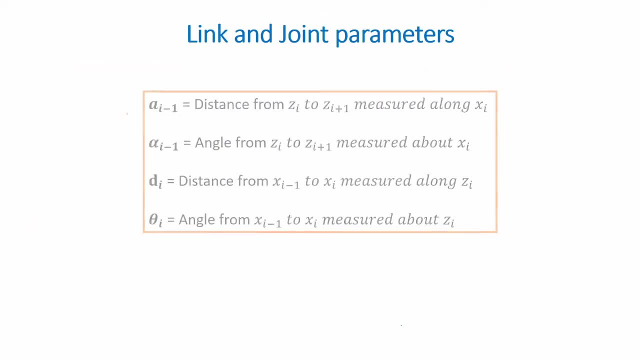 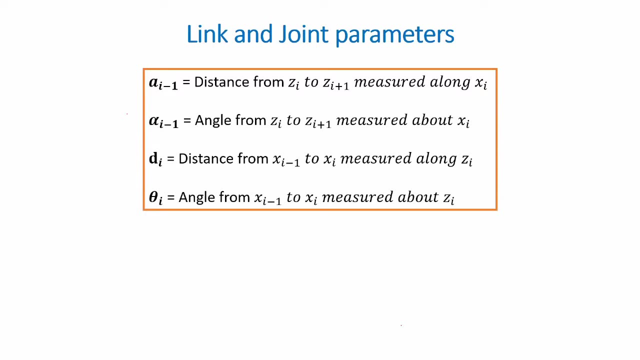 have a 0 T to I. so these are the four definitions that we will be using to find these four parameters. it is best to keep these definitions in mind and understand them, as it would make problem-solving much easier if you look at these definitions. like I mentioned earlier, only two axes are needed: the 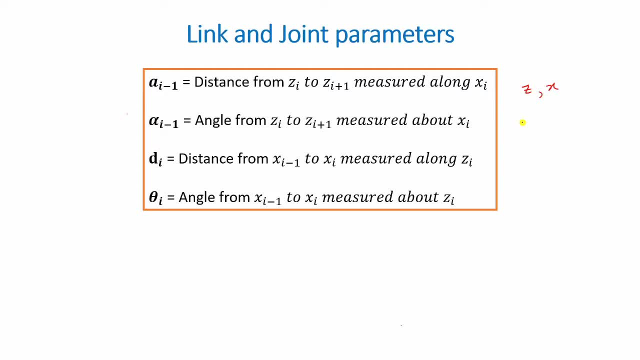 z-axis and the x-axis. in this case, for example, z I refer to the axis under question, while z I plus 1 will refer to the next joint axis and z I minus 1 will refer to the previous joint axis. using these four values, we can form a th table. 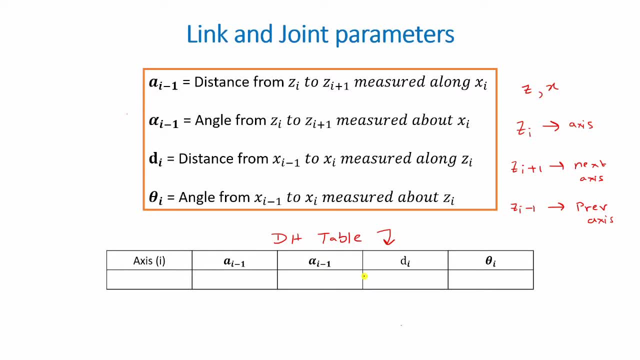 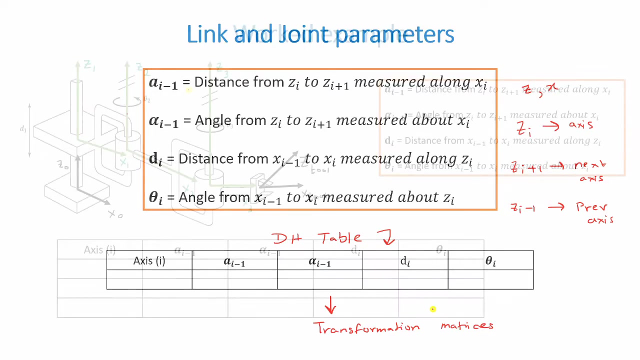 or Denavith- Hardenberg table, and using the values in a dh table, we can later find our transformation matrices using a particular equation. now, using these definitions are best understood through an example, so let's have a look at it. so, looking at this example, we assigned the frames. 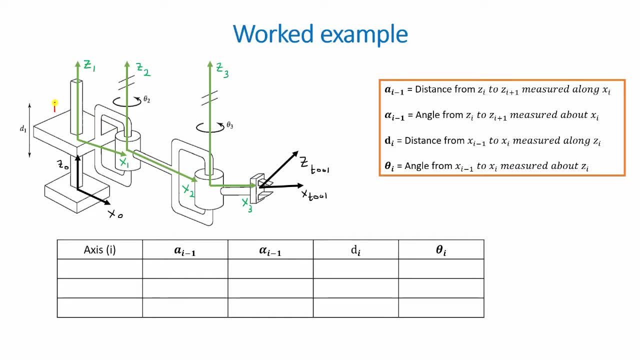 in the previous video by three patterns which are all marked with a number. so when a number is not, You can see there are three joints. you have a prismatic joint, a revolute joint and another revolute joint. So just by looking at the diagram you should be able to tell that the prismatic joint should 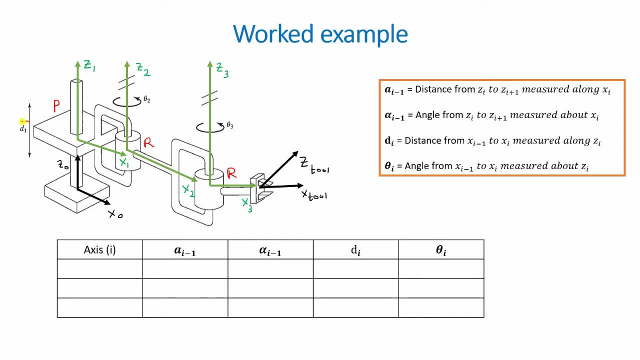 have some value for di, and that would actually be given by this variable here, d1.. The two revolute joints should have some value for theta, which would be theta2 and theta3.. The frame for the tool was already given in the question, while the base frame was assigned. 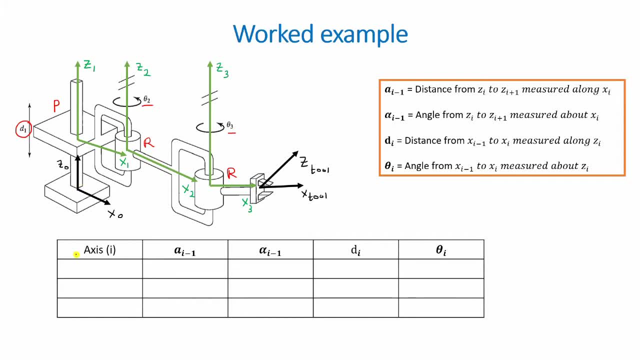 in relation to the first frame. Now, this would be our DH table, and the first step would be to identify the axes. So we have three axes: 1,, 2, 3, corresponding to our three joints. However, when setting the parameters for the DH table, we would always move from one frame. 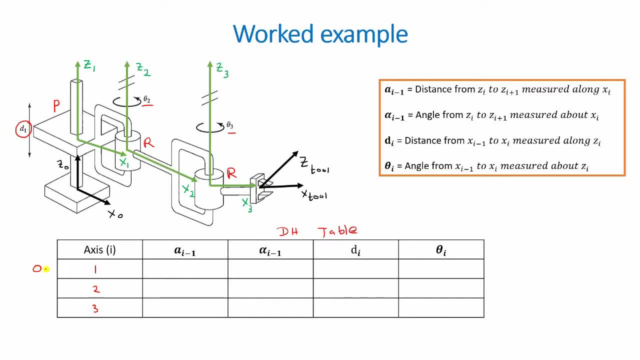 to another. So in the first case we will move from 0 to 0.. Then from 1 to 2 and 2 to 3.. So let's consider the first case, moving from 0 to 1.. Now for the first two parameters, a and alpha, i minus 1, i would be equal to 0. 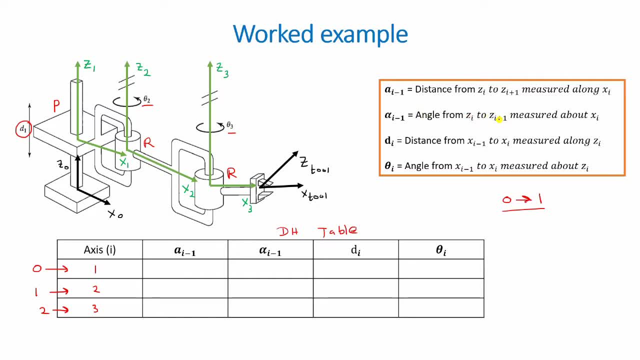 Because our z? i would be 0 and z i plus 1 would be 1.. But in the case of di and theta i i would be 1.. So our xi minus 1 can be 0. And our xi can be 1.. 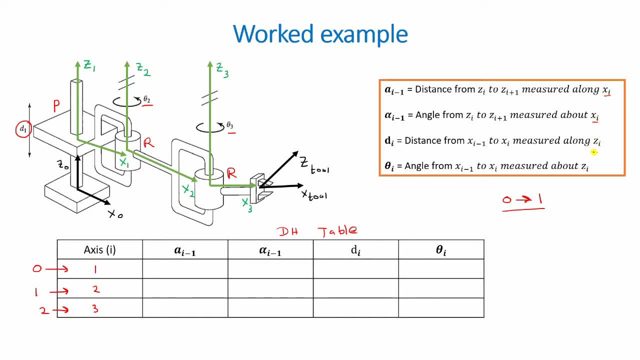 This is because we want to keep our xi's and zi's in relation. So let's have a look at it. For ai minus 1, we want the distance from z0 to z1 about our x0. So the distance between our z0 and our z1 is equal to 0. 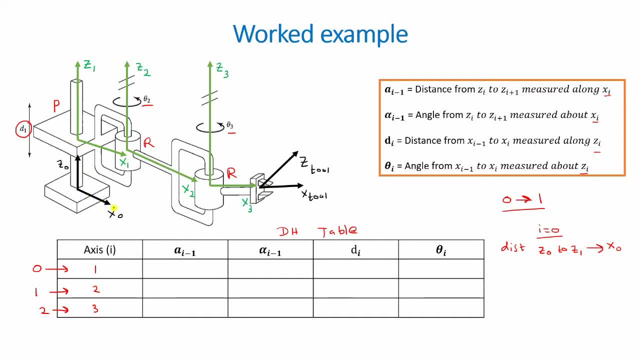 So the distance between our z0 and our z1 is equal to 0.. So the distance between our z0 and our z1 is equal to 0.. So we want to keep our xi's and zi's in relation along x0.. 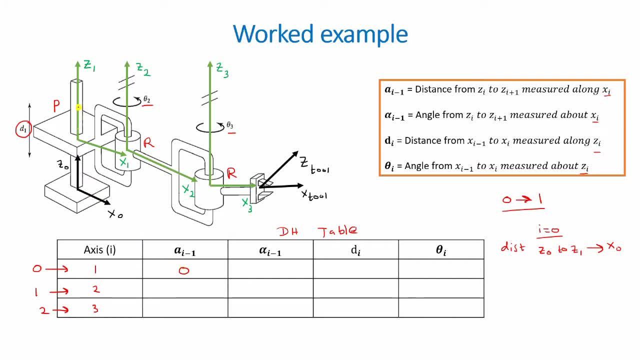 And you would see that this value is actually 0 because z0 and z1 are in line with each other, And so there is no displacement along the x axis. The second value, alpha i minus 1, looks at the angle between z0 and z1 about x0. 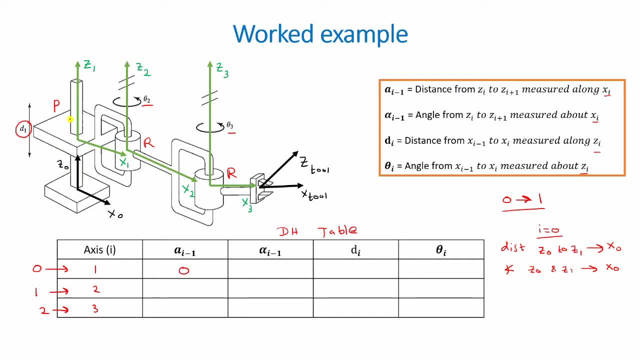 So this is the angle. z0 has to rotate to align with z1 about x0 axis and as they are both pointing vertically upwards and in line, this angle is 0. now I becomes equal to 1 again. we want the distance for DI between our x, not to x1 about z1. so the distance between my X 0. 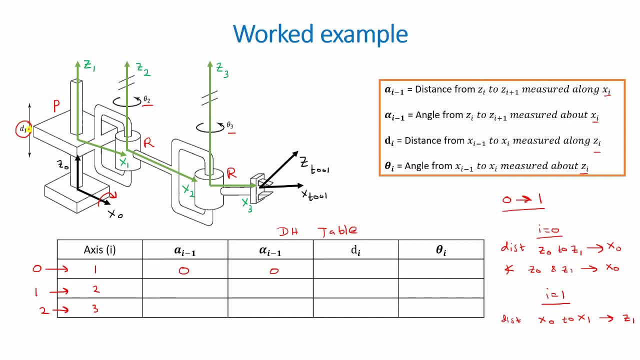 and X 1 about z1 would actually be D 1 because it is a prismatic joint. well, as the angle from X 0 to x 1 about z 1 would be 0, and this is because x0 and x1, so how we can rotate our x0 to match up with x1 about z1. so 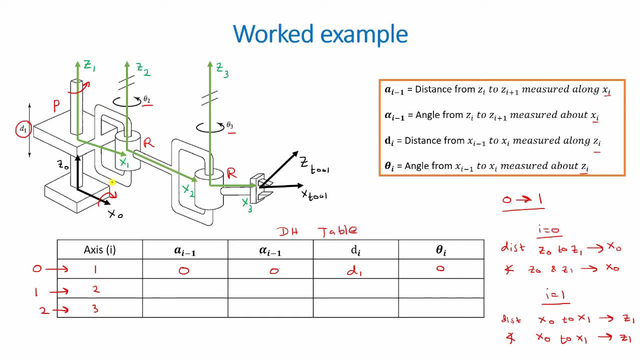 the rotation would be here. they're both in line and both pointing in the same direction, so the angle would be 0. there would be no rotation around z1. now let's look at frame 1 to 2. right, so now considering frame 1 to 2. so for the first two values of i would be equal to: 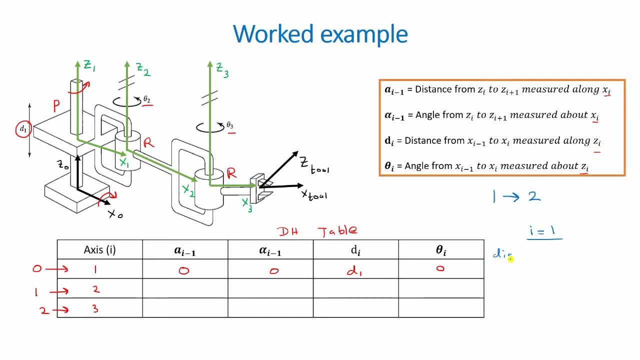 1. so our ai minus 1 is going to be equal to 2. so for the first two values of i would be 1. would want our distance from z1 to z2 about x1, the distance between z1 and z2 in the direction. 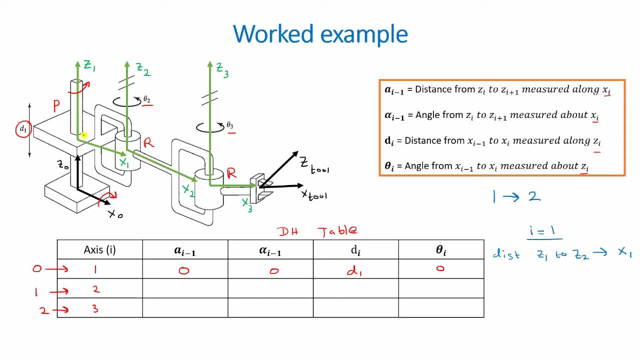 of x1 and this would actually be the length of the link from z1 to z2. so we can imagine a parameter or the length of the link to be l1, and that would be your ai minus 1, then the angle between z1 and z2 about x1. so this is the angle: z1 must rotate to match up to z2. 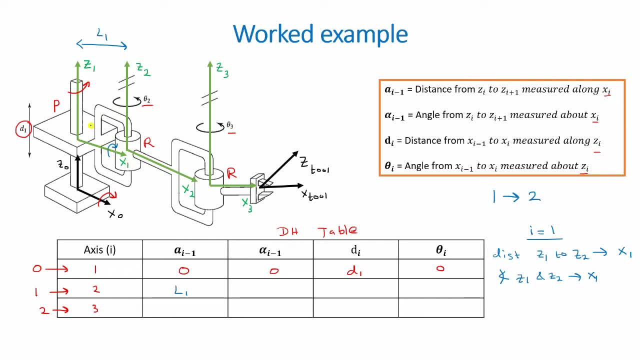 if rotated about x1's axis. as both z1 and z2 are parallel and pointing in the same direction, this angle is 0. now we look at i equals 2 for the final two parameters for di. we want the distance between my x1 to x2 about z2, the distance between my x1 and x2 in line of z2. so x1 and x2 are both. 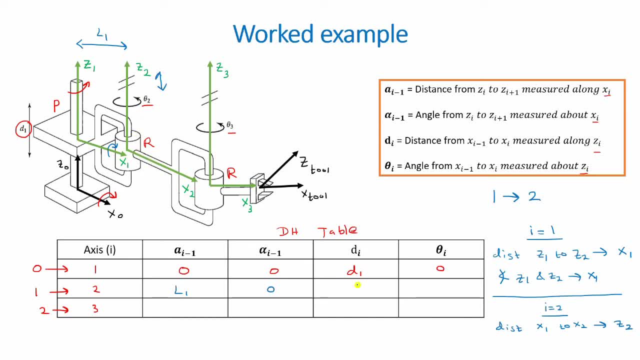 on the same plane. there is no vertical displacement. so this is 0 for theta. i point Finding x1 and z2. so the value of z low of theta in length of by about 1 world, the angle between x1 and x2. at about 0 left, the angle x1 will be theta 2holding angle between x1 and x2, z2. so how will your value of Angle Bag? and this angle would be Theta 2 And this angle is Theta 2, andas, you can see, this is a Revolute joint, hence it has a 0 Di but a theta value than before we were looking at a prismatic fronts. so it has some di value, which is di value, but zero. tryin 8 μια. as by возду oya, value which is d, 1, but zero only. as previously we were looking at prismatic points, we have some di value which is zero and 360 to be just d, and this is. however, this value contains a 0 kinda right and i will use this collaboration to substitute: is thatement here?